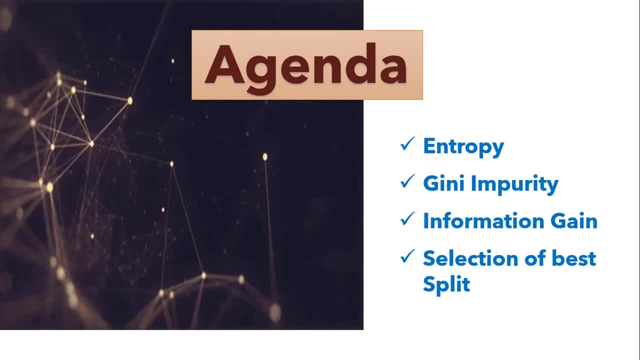 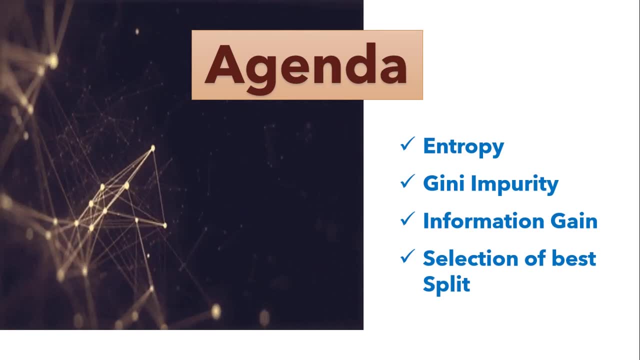 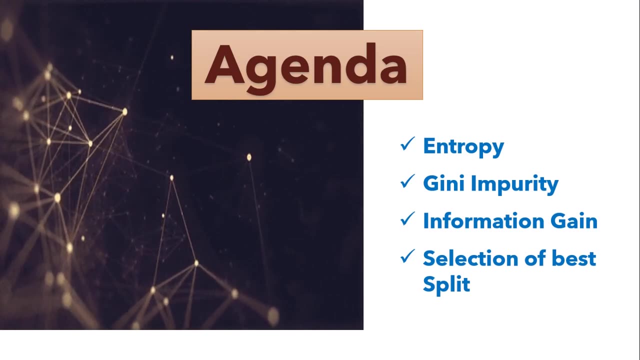 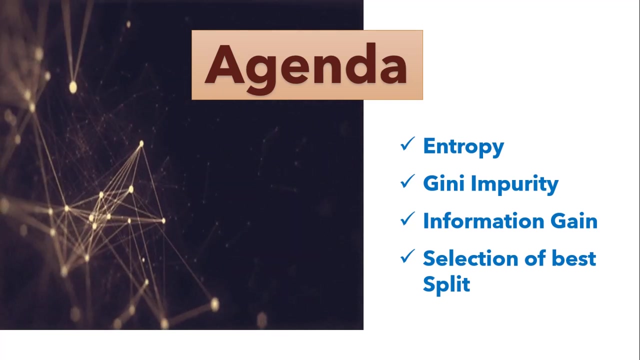 So, guys, I have divided this video in three parts and today our focus will only be to understand basic intuition of entropy, Gini impurity and information gain. We will see how can we solve classification and regression problem using decision tree in upcoming sessions. Alright, so let's quickly start understanding what is decision tree. 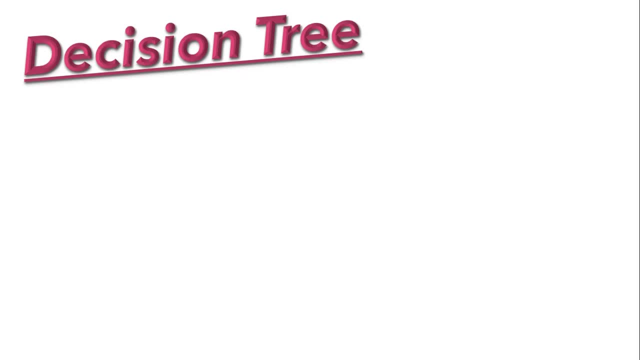 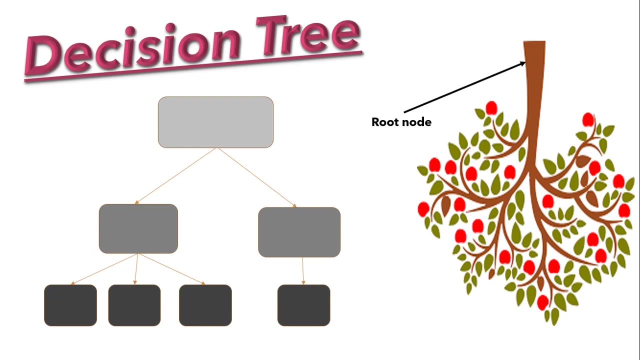 So decision tree typically starts with a single node which branches into possible outcomes. Each of those outcomes leads to additional nodes which branches off into other possibilities. So in simple words, we try to create a tree like structure where we can consider stem of the tree as root node, its branches as different conditional attributes, and fruit. 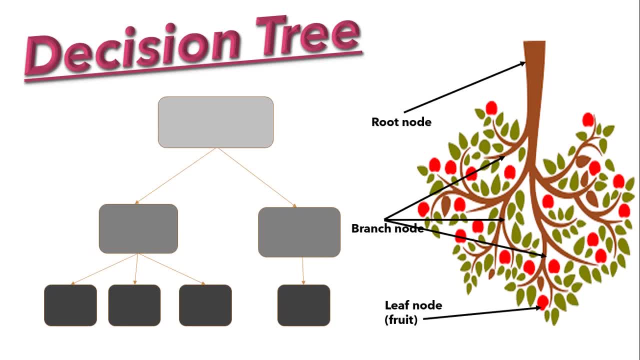 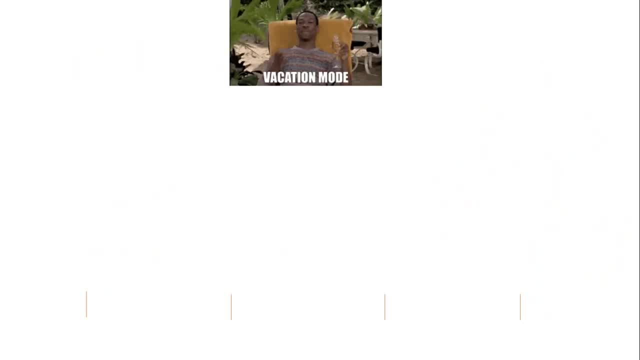 as final result. So let's understand this first. Let's start with one example. So suppose you want to go out for a vacation, but you are not sure where should you go. So what you will do is you go to your friends and ask them to suggest you any place, And 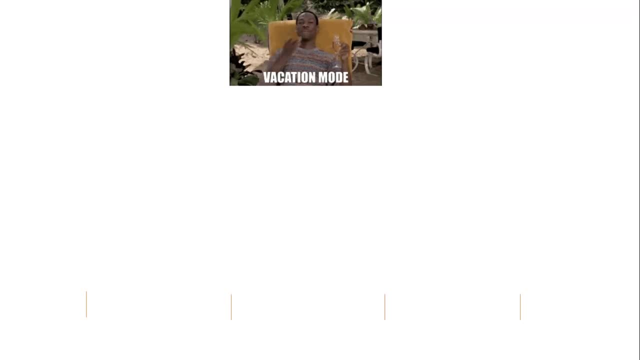 then you will categorize those places with some conditions. Let's say your friend A is suggesting you to go to Goa and friend B is suggesting you to go to Uttarakhand. Now you will have a look on all possible conditions to decide which place you want to go to. So 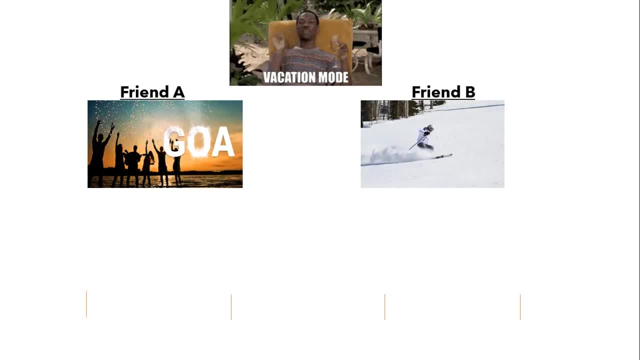 you won't be able to decide, to decide any of the places for your vacation. Now, let's say your conditions are constrained to whether you want to go for a hilly area or beaches, Then, whether you have a budget of more than 15k bucks or not, Then your third. 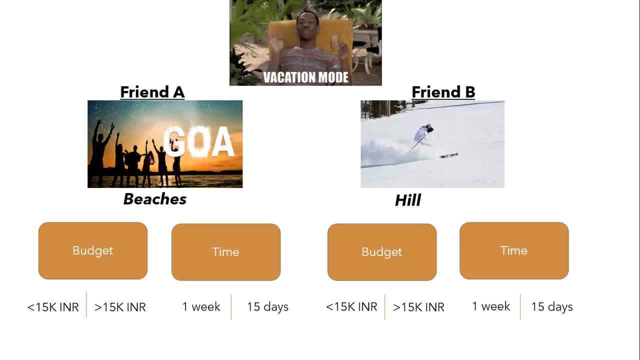 condition will be like how many days you have to spend for this trip. Once you list out all these conditions, you will be able to prioritize where should you go for vacation. So, basically, we are trying to create a standard daily vacation structure based on the conditions which we 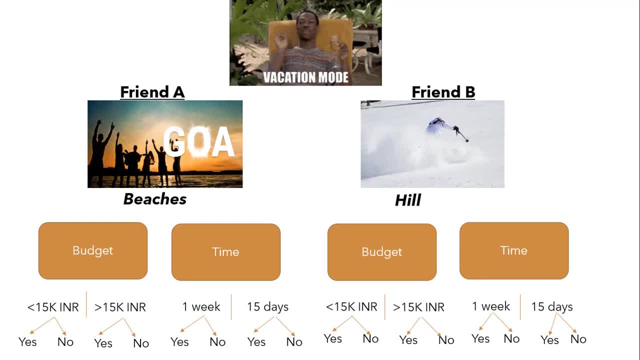 are able to make. So the first condition is: you want to go to your friends, and where should tree structure to reach to our final outcome, as you can see on the screen? Same we do in case of building decision tree algorithm, but with algorithmic approach. that 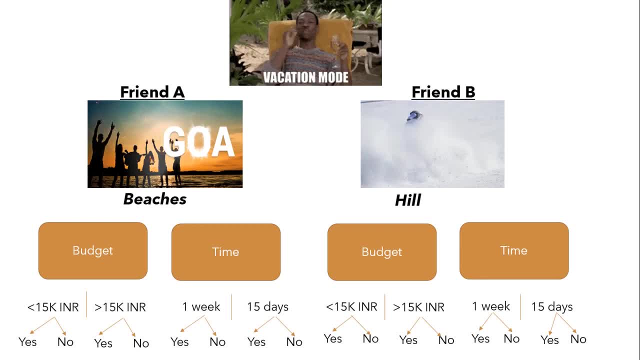 identifies ways to split a data set based on different conditions. So now I can say that the decision rules are generally in form of if-else statements. So let's understand how can we create these splits or branches, and how can we say which branch is best. 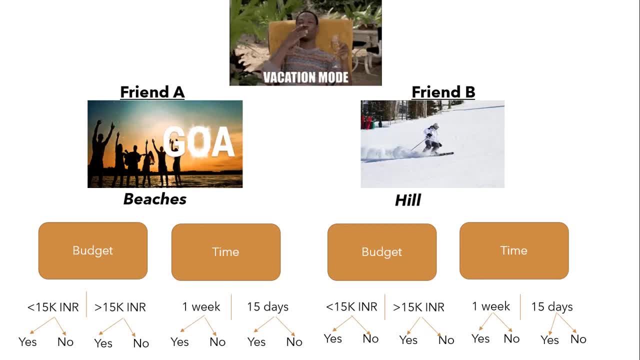 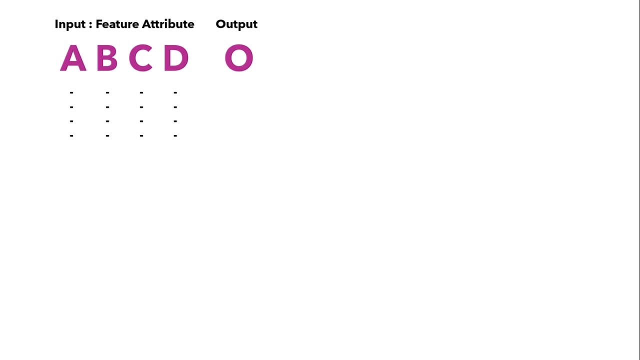 So, guys, for answering this, we have some metrics, that is, entropy, information gain and Gini impurity. Let's understand these one by one. Let's say we have some feature attributes, that is, A, B, C, D as input and O as output. 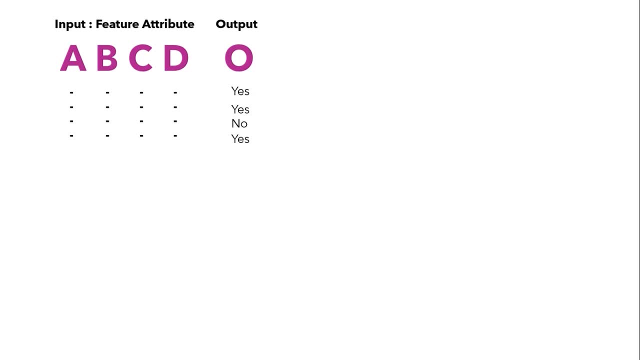 which is having either yes or no values. So, based on different attributes, we have to predict whether output will be yes or no. So, Okay. So according to ID3 algorithm, our first step is to select the right attribute for splitting. So for considering which attribute should we use to split the tree, we use entropy function. 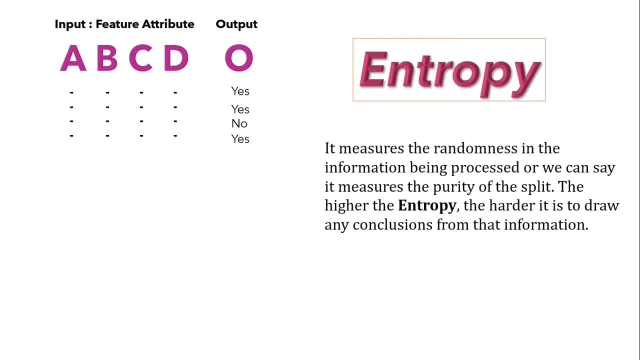 See, if we don't select the right attribute, then our tree will go till the much depth and increase the time complexity as well. So, guys, entropy measures the purity of split. Let's say my root node has 7 yes and 5 no, and when I split this into branches and come to node B, I got somewhere. 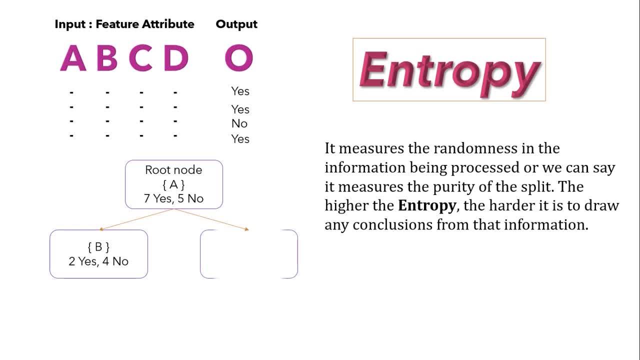 around 2 yes and 4 no, and at C node I got 5 yes and 1 no. So, guys, you can see that the split is not pure subtree, as it contains both yes or no, And pure subtree basically means that either we should be getting yes or no. 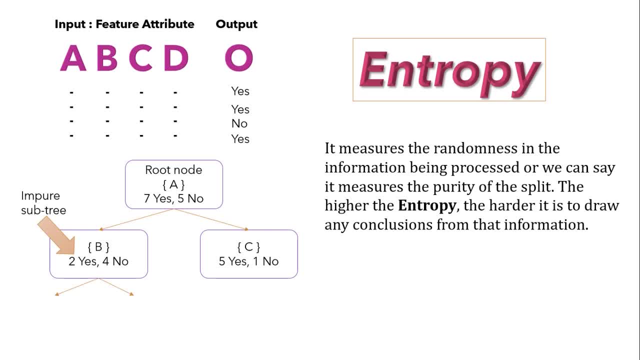 So based on this, again, I will split this subtree. So node D will be 2- yes, 0- no. and node E will be 0- yes, 4 no. Same we will do for node C. So here you can see that this can be categorized as pure subtree, as at this layer. 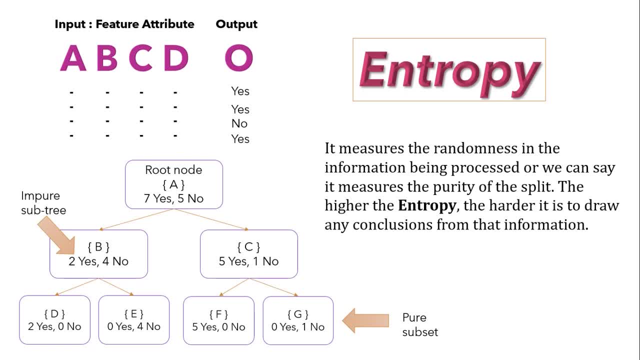 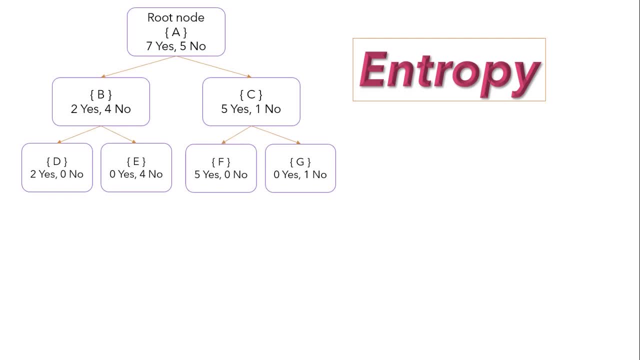 we have either yes or no component with us. So, guys, for finding out the best split with pure subtree, we need entropy function. So, guys, we have formula for entropy as sigma: i equal to 1 up to c minus pi, log base 2 of pi. 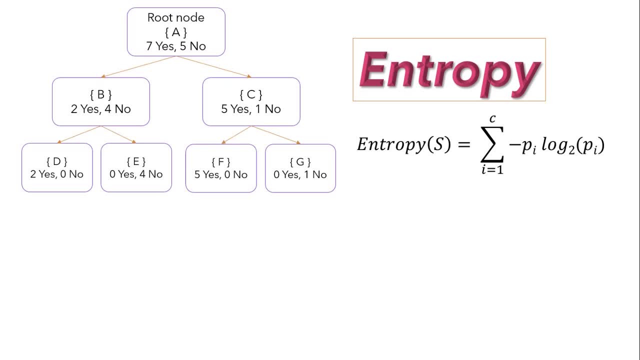 Let's understand what is p over here. If I talk about node A, then p for yes can be considered as probability of yes over sum of probability of yes and probability of no. So now we have to compute the entropy for both the nodes for deciding whether we can go to node B. 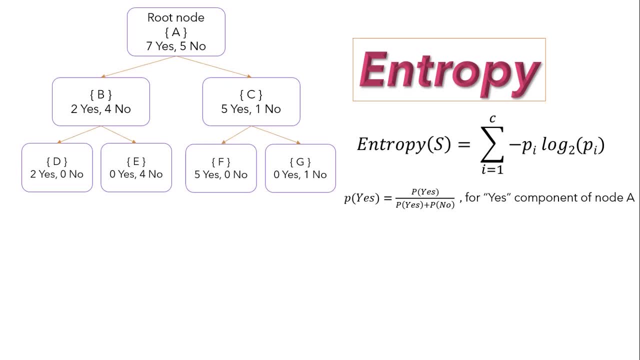 or node C. So let's calculate the entropy for node B first. So here we have 2 yes and 4 no. Let's substitute these values to equation Negative of 2 over 6.. So here we consider our denominator as sum of probability of yes and probability of no. 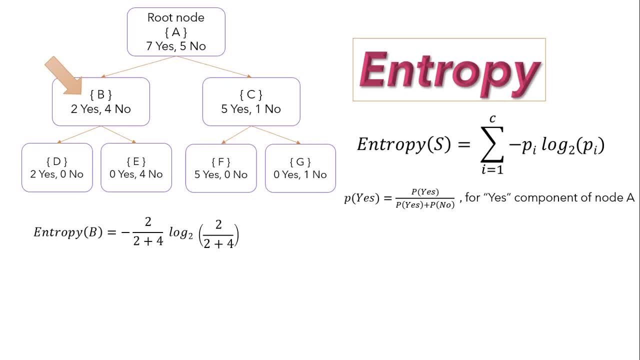 As I told you earlier. So negative of 2 over 6 into log base: 2 of 2 over 6 minus 4 over 6.. So here we consider our denominator as sum of probability of yes and probability of no. Here we have 4 no, and sum of probability of yes and probability of no is 6.. 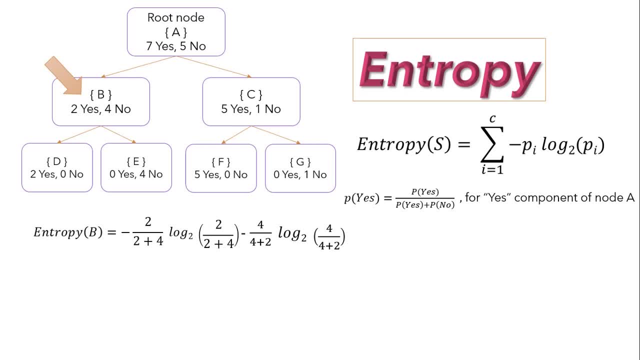 So minus 4 over 6 into log base 2, 4 over 6.. So after computing this we can get entropy for this node as 0.92 bits. By same mean we can compute entropy for node C as 0.65 bits. 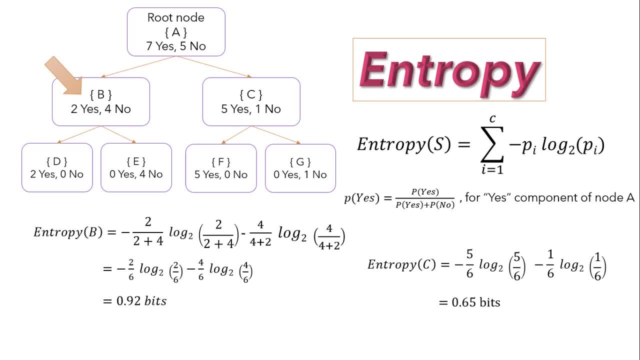 So, guys, one thing to add here is that entropy ranges between 0 to 1. We consider zero as pure subtree, whereas one can be considered as worst scenario or most impure subtree when both yes and no are equal in number. So each time when we compute entropy, we consider the value which is more closer to zero. 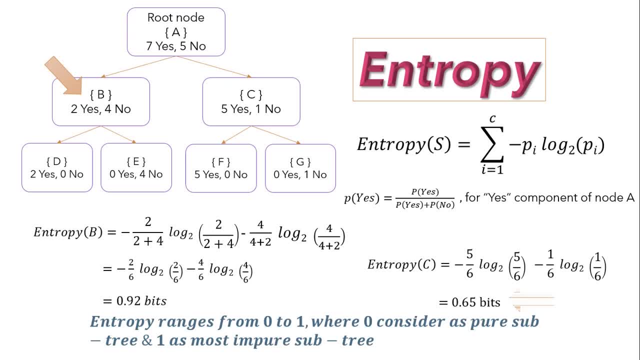 So, guys, now we can say that node C is having less value, so we can continue with node C. But this is not it Here. We should also consider that after splitting this node, we may also require some other attribute to reach the leaf node. 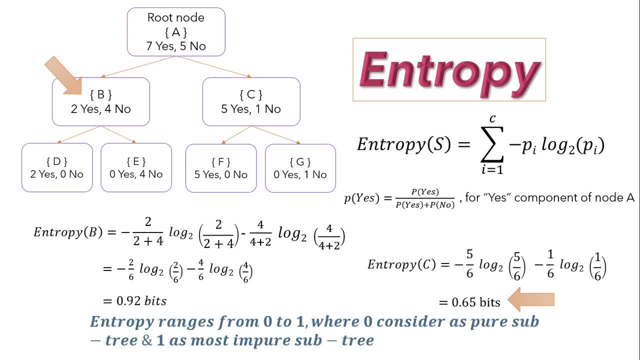 So we have to take entropy of those attributes too, And after adding up all attribute of a particular split till leaf node, then only we can justify that which split is best for our use case. So how can we achieve this? So, guys, we have new matrix known as information gain. 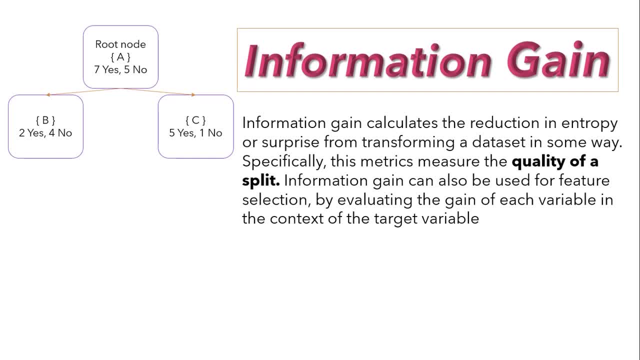 It combines all the entropy together till the leaf node. So formula for information gain is entropy of S minus sigma of V. two values into S of V over S into entropy of SV. So here entropy of S we have just find out for each node. 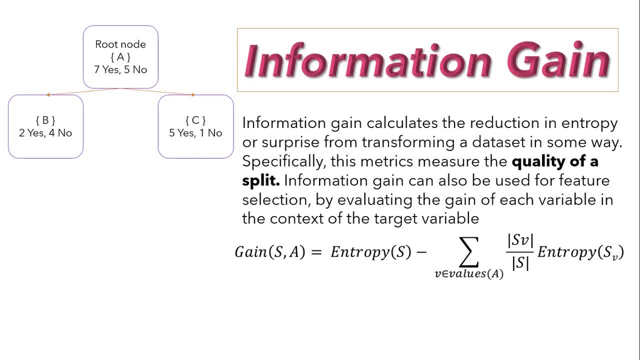 And S of V is our subset after splitting. S is total subset and entropy of S of V is total subset. Entropy will be after splitting. we want to calculate the entropy for particular subset. I know this looks complicated to you guys, but we will understand this with one example. 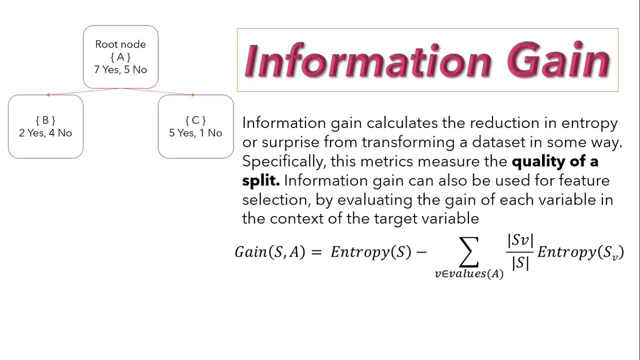 So again I will consider the same split, what we have used for understanding entropy. So here node A is splitting into node B and node C, where node A has 7 yes, 5 no, node B has 2 yes, 4 no And node C has 4 no. 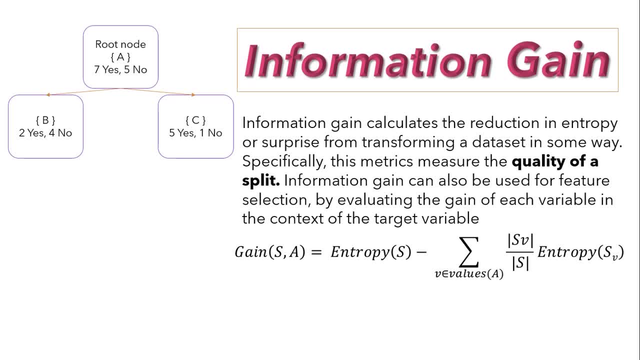 And node C has 5 yes, 1 no. So according to the formula, first we have to calculate entropy of S, which is nothing but the entropy of node A, that is, root node. So I will apply the same entropy function for this and I can get it as 0.97. 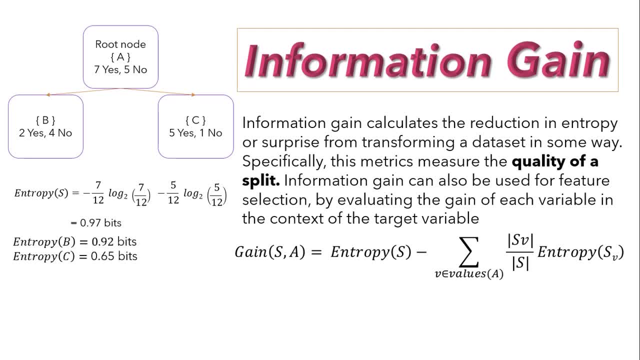 Then we will compute entropy of node B and node C, which we have already calculated as 0.92 and 0.65.. So here entropy of node B and node C will be considered as entropy of S of V. Now let's substitute these values to the equation as shown on the screen. 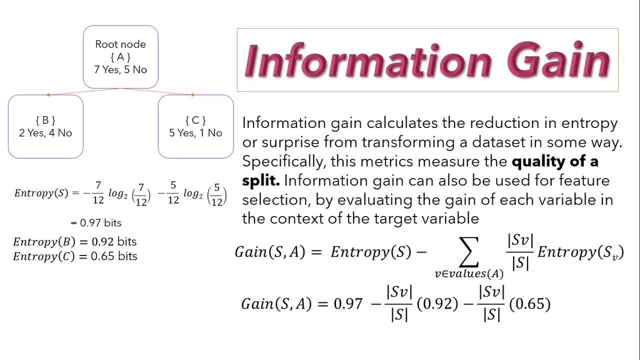 So, guys, here we have to substitute S of V over S. Let's understand what is this. If I talk about node B, then S of V will be total number of components. that is, 2 plus 4 is equal to 6.. And S is total subset. 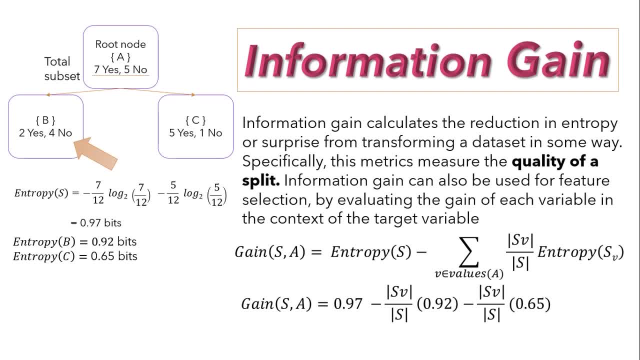 So here we have to substitute S of V over S. Let's understand what is this. Total subset, that is, 5 plus 7, is equal to 12.. So we can substitute S of V over S for node B as 6 over 12.. 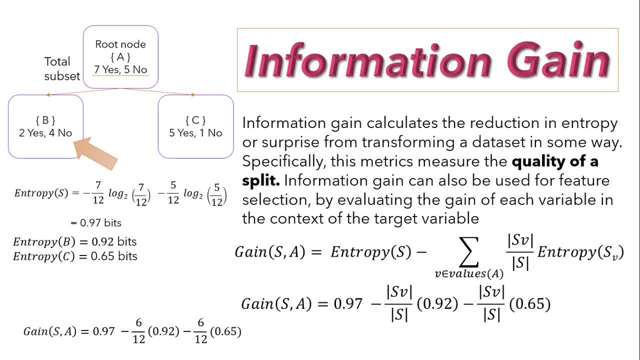 And for node C, S of V over S will be again 6 over 12.. Let's calculate 0.97 minus 6 over 12 into 0.92 minus 6 over 12 into 0.65 and find out the information gain. 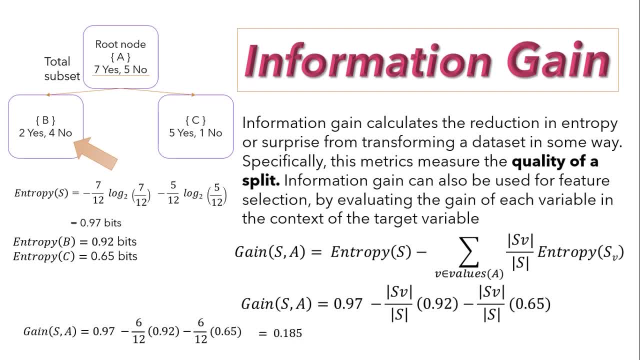 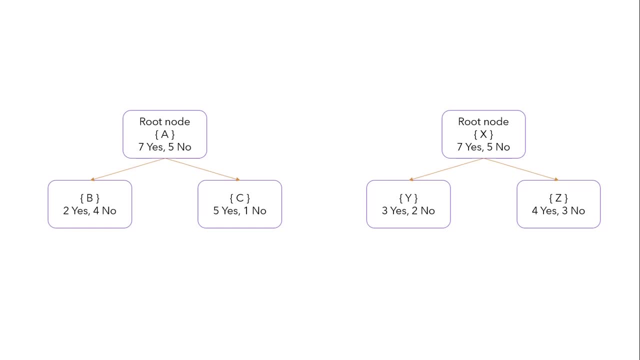 So we will find out the information gain as 0.185.. Now let's understand what it denotes. So suppose we have two splitting mechanism with us, one, what we have just calculated, and another one as shown on the screen. So we will find out the information gain for this as well. 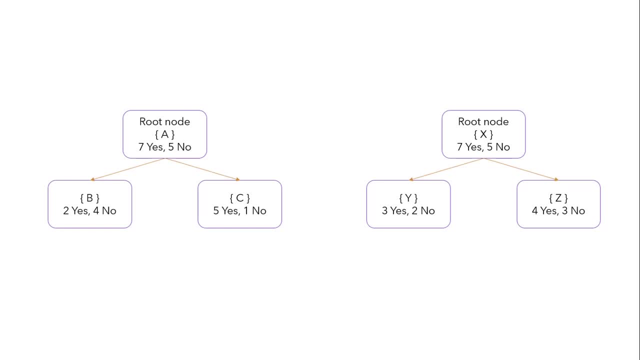 Then we will compare the two and we will only consider the splitting mechanism which is giving us the higher information gain between these two. So, guys, here we have to substitute S of V over S for node B. So, guys, this is very important to remember: how to calculate information gain while considering. 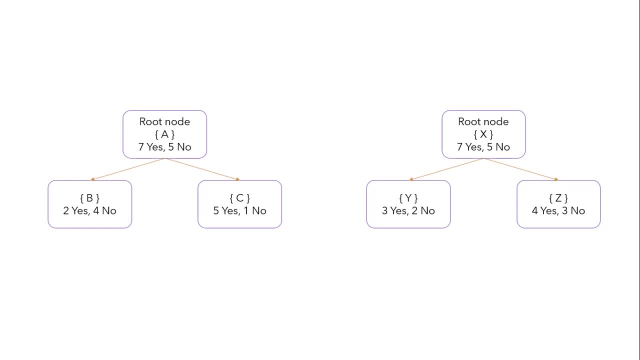 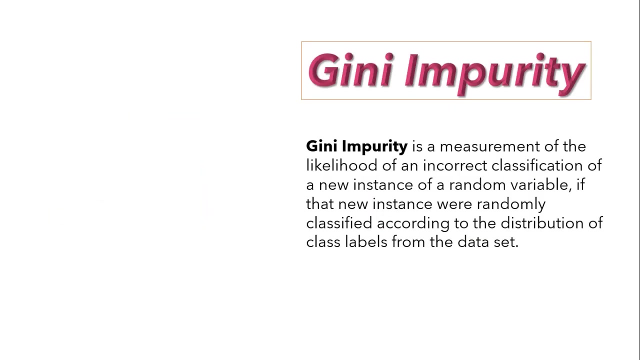 entropy, As we have python packages with us for automatically calculating the splits. but you should understand the inner functionality of these mechanisms. So, guys, we have one more matrix and that is Gini impurity. Let's understand that as well, as we can either use entropy or Gini impurity- both gives us. 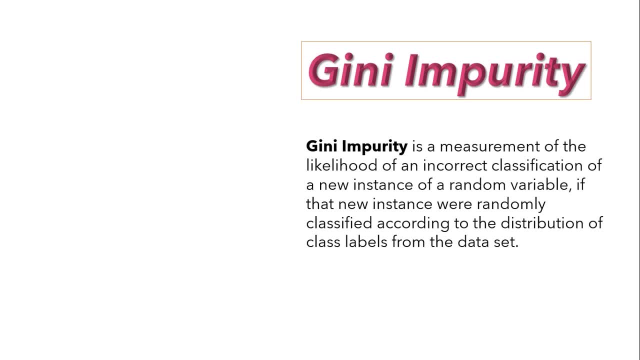 the measure of purity, But with different parameters. So we have already known the formula for entropy and we have seen how to calculate entropy for a particular node or attribute. So, guys, formula for Gini impurity is 1 minus sigma of p square, where p is probability of. 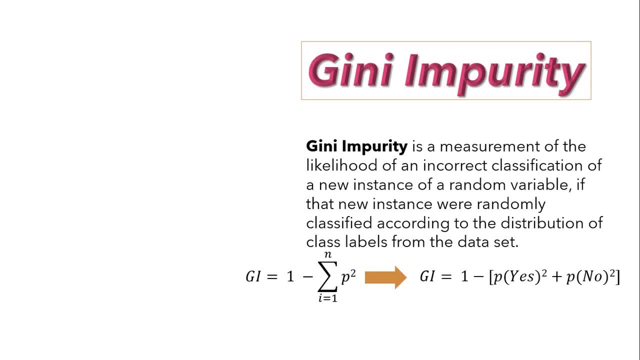 yes, plus probability of no. Let's understand this with one example. So, guys, we have calculated the entropy for node C as 0.65.. So, guys, we have calculated the entropy for node C as 0.65.. Let me substitute the values in Gini impurity equation for you, So that will be 1 minus P of. 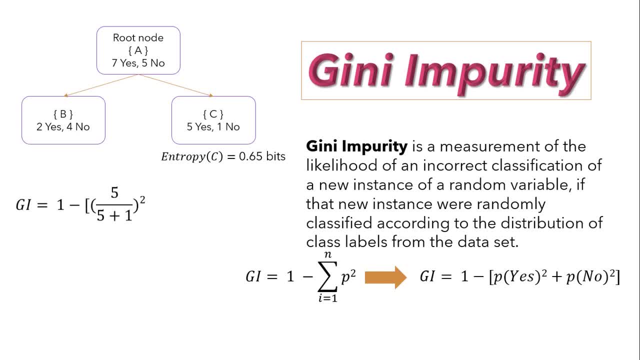 s, and here P of s, will be square of probability of yes over probability of yes plus probability of no, and this will be square of 5 over 6 plus probability of no and probability of no. will be square of probability of no over probability of yes plus probability of no, and this is calculated.